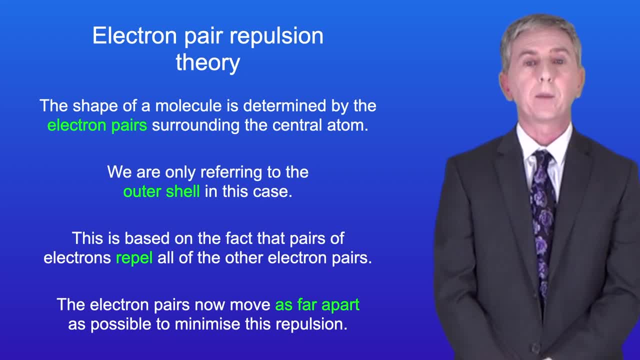 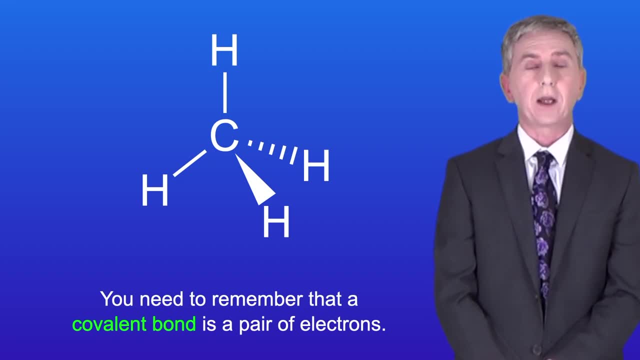 electron pairs. The electron pairs now move as far apart as possible to minimize this repulsion. Now, we've been referring to pairs of electrons, but you need to remember that a covalent bond is a pair of electrons. Now, one thing I need to point out is that in this video, we're only looking at 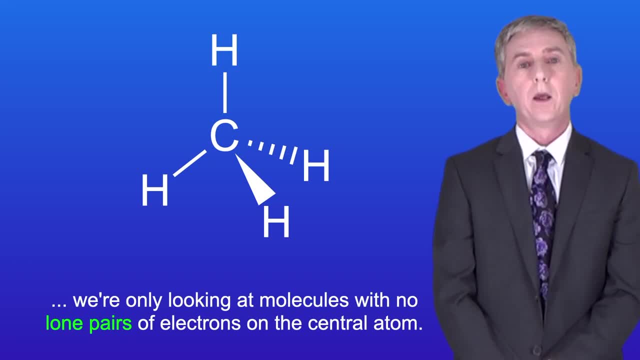 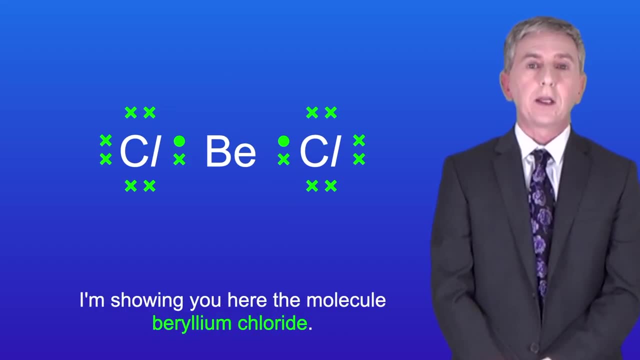 molecules with no lone pairs of electrons on the central atom. We'll be looking at how to deal with lone pairs in the next video. OK, let's look at a simple example. I'm showing you here the molecule beryllium chloride. 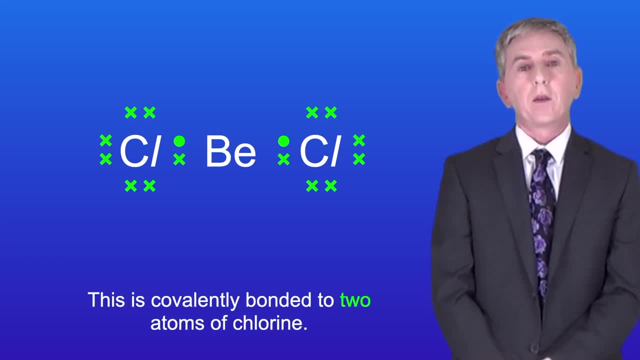 In this molecule the central atom is beryllium. This is covalently bonded to two atoms of chlorine. So this means that we've got two electron pairs around the central atom. These two pairs of electrons repel each other and move as far apart as possible. Now, the furthest that they can move apart is in a 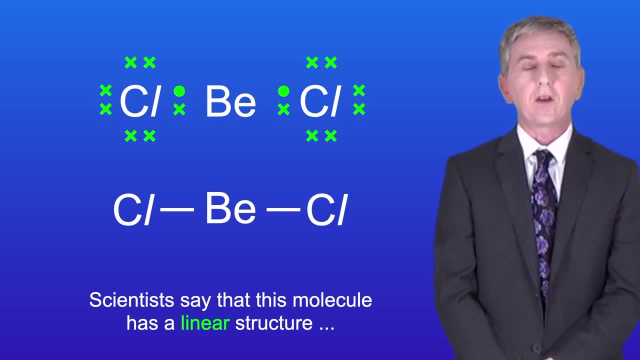 straight line like this. Scientists say that this molecule has a linear structure, in other words, a straight line, And the angle between these two bonds is 180 degrees. Here's another linear molecule. This is carbon dioxide. Now, this illustrates a really important point. 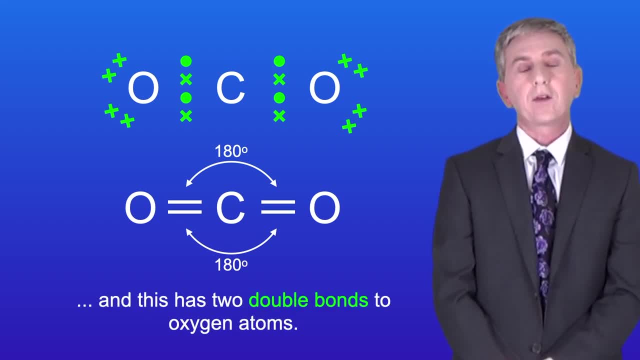 As you can see, the central atom is carbon and this has two double bonds to oxygen atoms. When looking at multiple bonds, such as double or triple bonds to determine the shape of the molecule, we treat a multiple bond as a single bonding area. In other words, we treat a double bond the same way. 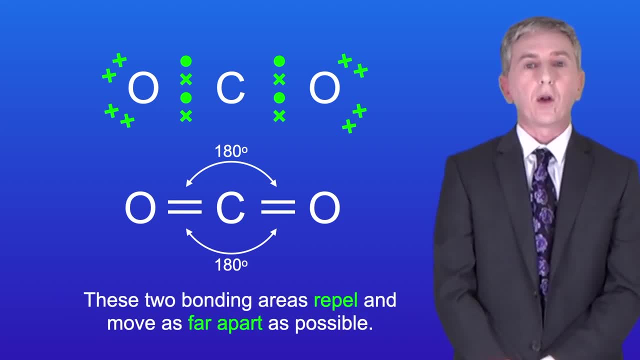 we treat a single bond, So these two bonding areas repel and move as far apart as possible. And again, in this case the angle between the bonding areas is 180 degrees. So you need to learn that if a central atom has two bonds or bonding areas, then it will have a linear shape. 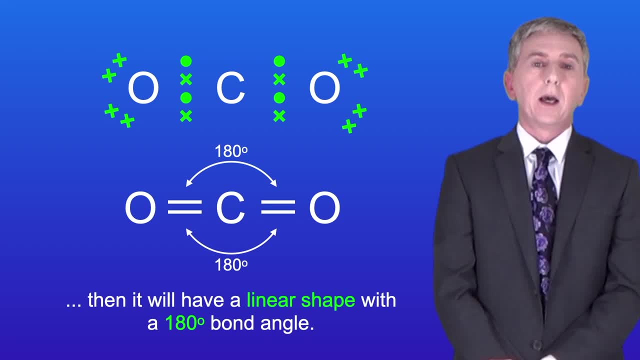 with a 180 degree bond angle. However, this is not the case if the central atom has a long pair of electrons And, as I said, we look at those in the next video. In the next section we're going to look at other things. 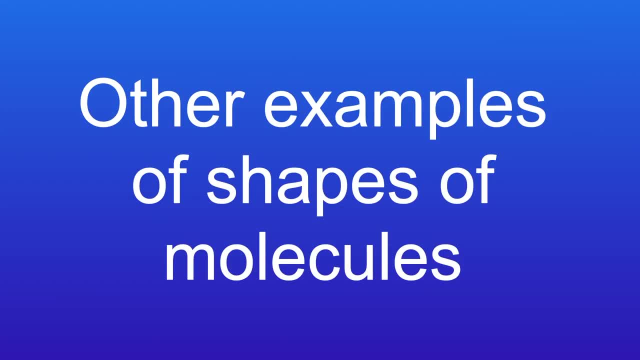 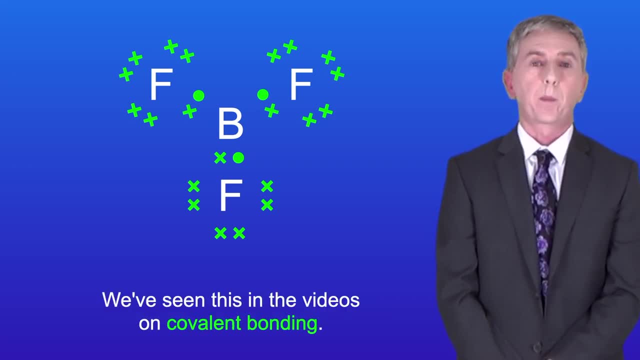 and other examples of the shapes of molecules. OK, this molecule is boron trifluoride and we've seen this in the videos on covalent bonding. This has a central boron atom bonded to three fluorine atoms. Again, the electron pairs in these three covalent bonds repel and move apart as far as possible. 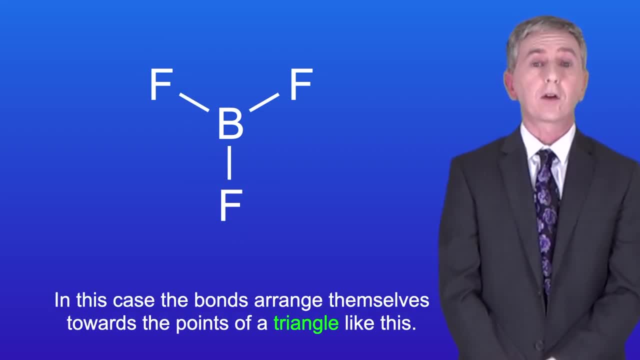 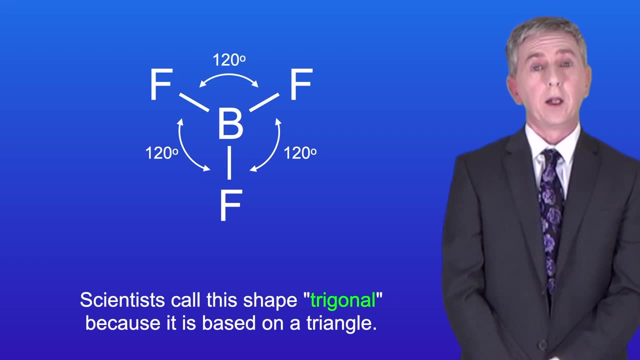 In this case, the bonds arrange themselves towards the points of a triangle like this, and the bond angle between them is 120 degrees. Scientists call this shape trigonal because it's based on a triangle. Now, if you viewed the molecule from the side, you would see that it's flat. 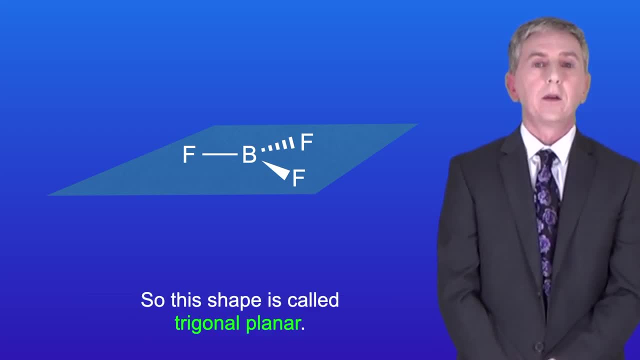 Scientists call this planar, which means flat. So this shape is called trigonal planar And you'll see this whenever you've got a central atom with three pairs of bonding electrons around it. as long as the central atom has no long pairs of electrons, 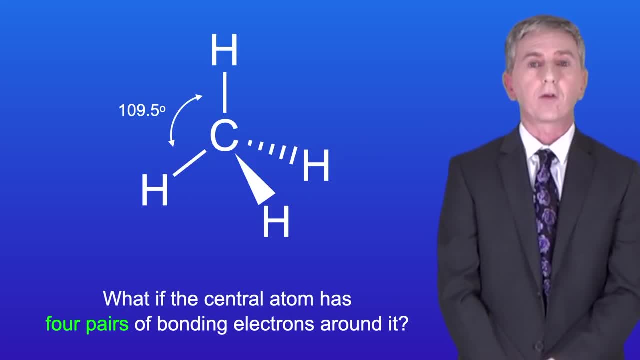 OK, what if this central atom has four pairs of bonding electrons around it? Well, in this case we've got a tetrahedral molecule, and a good example is methane. All of the bond angles in tetrahedral molecules are 109.5 degrees. 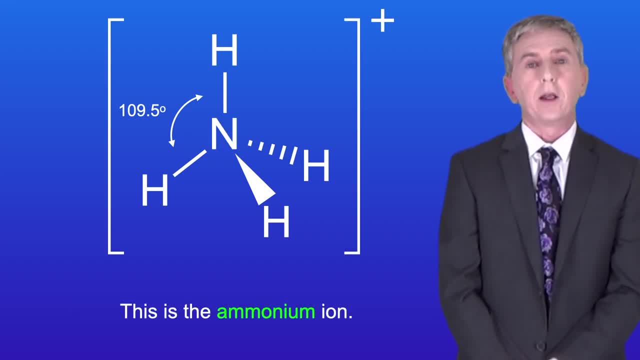 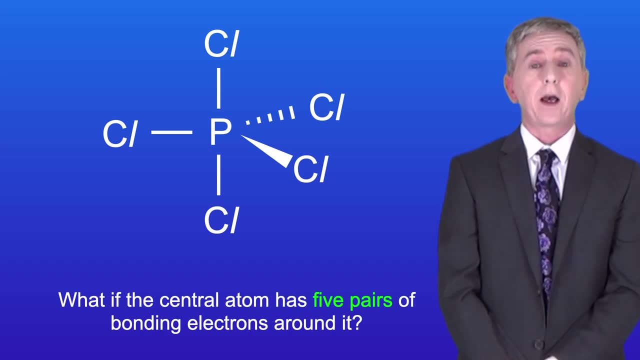 Here's another tetrahedral molecule. This is the ammonium ion, And again, the bond angles are all 109.5 degrees. OK, so what if this central atom has five pairs of bonding electrons around it? A good example is phosphorus pentachloride. 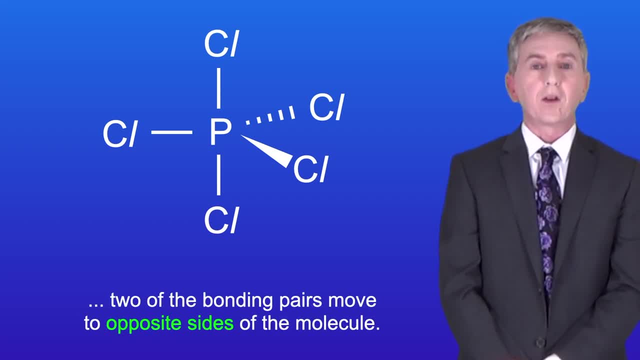 Well, in this case, in order to minimize repulsion, two of the bonding pairs move to opposite directions. They move to opposite sides of the molecule, and we can see these here. The other three bonding pairs now take up a central position, lying on the same plane. 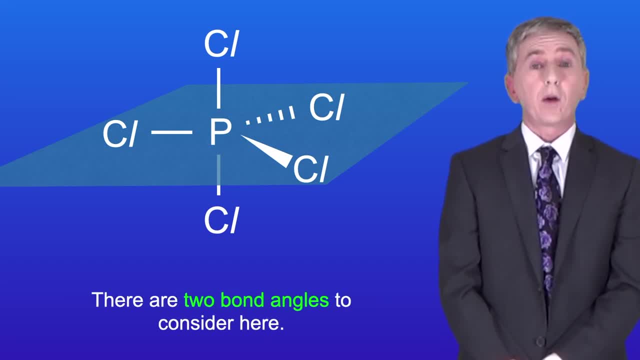 and they spread themselves out as far as they can. Now there are two bond angles to consider here. The bonds pointing up and down are at 90 degrees to the central plane, whereas the angle between the bonds lying on the central plane is 120 degrees. 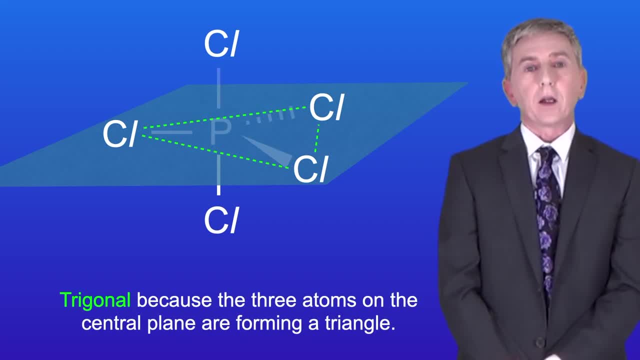 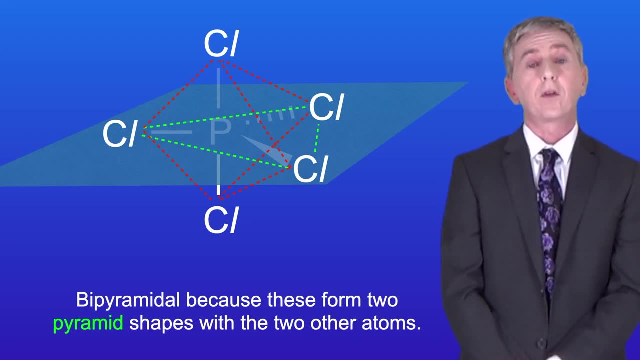 Now this shape is called trigonal bipyramidal. In other words, the three atoms on the central plane are forming a triangle And bipyramidal because these form two pyramid shapes with the two other atoms. So here's the pyramid above the plane and here's the pyramid below. 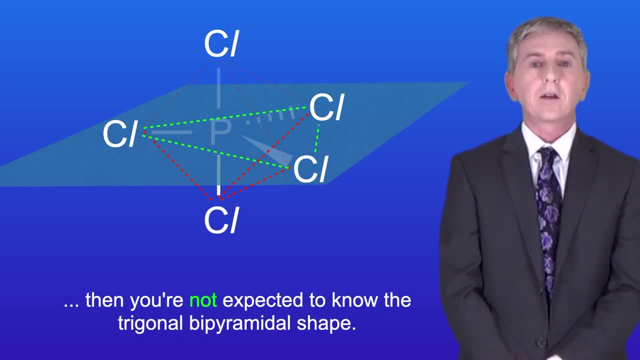 Now I should just point out that if you're following the OCR spec, then you're not expected to know the trigonal bipyramidal shape. However, I'd recommend that you're aware of it in case it appears in a question where you have to apply your knowledge. 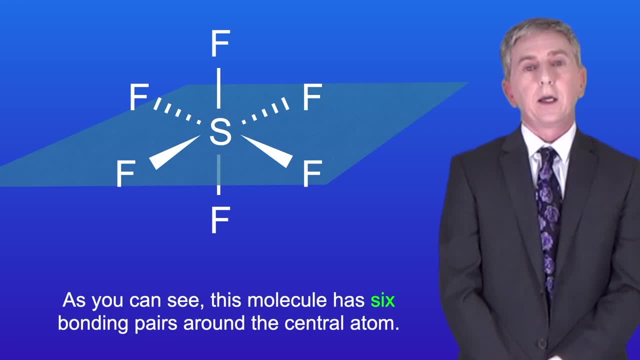 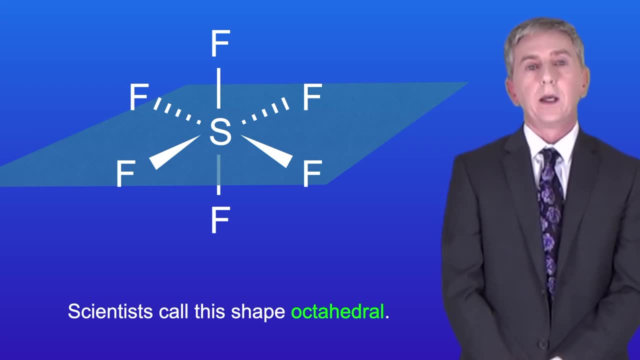 OK, I'm showing you here the compound sulfur hexafluoride. As you can see, this molecule has got six bonding pairs around the central atom. Scientists call this shape octahedral. Again, we have a bonding pair above and below the central plane. 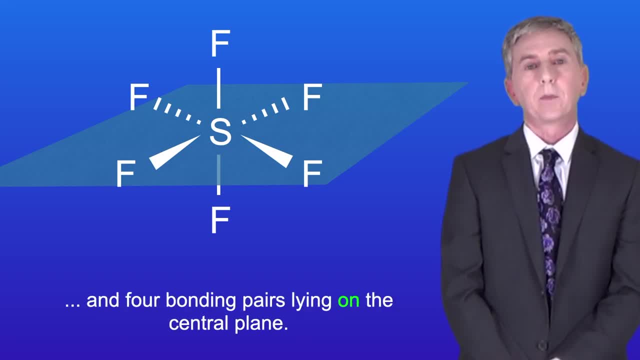 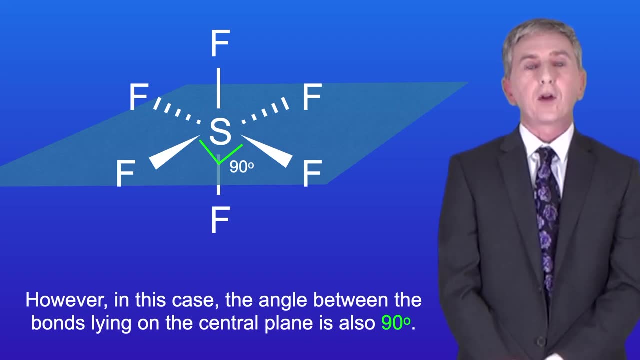 and four bonding pairs lying on the central plane. Just like before, the bonds pointing up and down are at 90 degrees to the central plane. However, in this case, the angle between the bonds lying on the central plane is also 90 degrees. 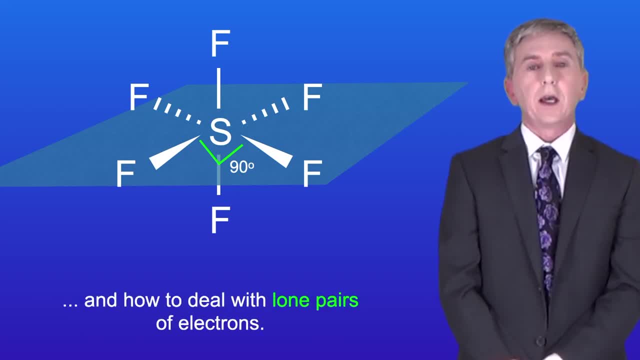 In the next video we're going to look at the shapes of ions and how to deal with lone pairs of electrons. Thank you for watching. 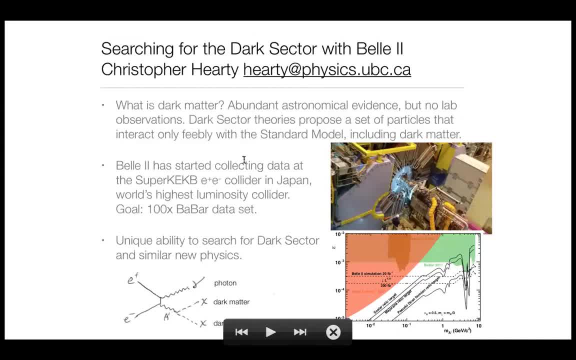 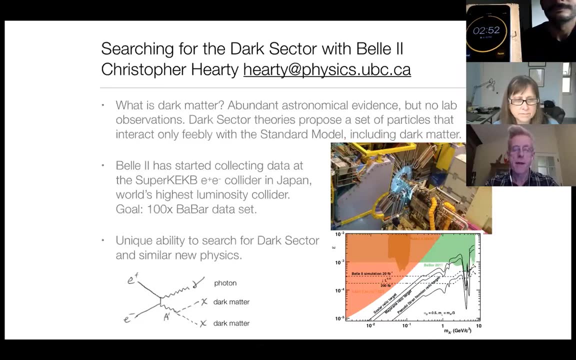 Our next speaker is Chris Hardy. My name is Chris Hardy and I work on BELL2, which is a large international collaboration. It's a particle physics experiment located at the KEK laboratory in Japan. It operates at the super KEKB E plus- E minus collider, which is the world's highest luminosity. 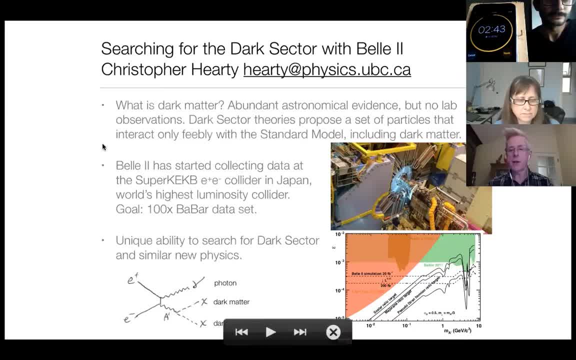 collider. You can see the large detector here. It's actually not that large by the standards of particle physics, but in absolute sense it's large. Now BELL2 has a very large physics program. What I'm interested in is dark matter. Now all. 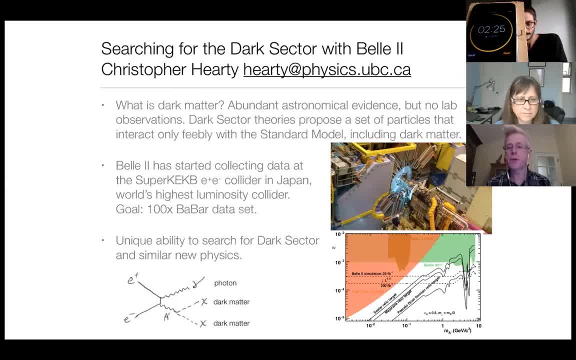 have heard, undoubtedly about dark matter, but there's abundant astronomical evidence but no lab observations to give us any hint as to what it is Now one. there's a lot of theories, of course, to explain it, but a recent area that's very. 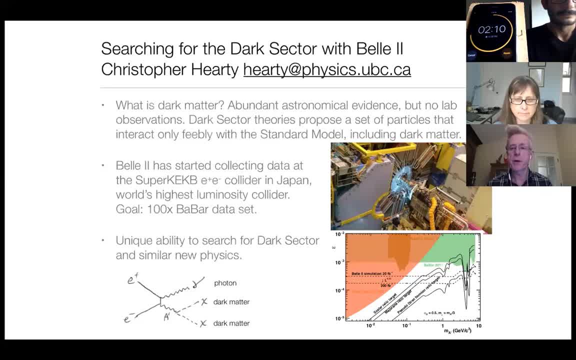 hot are called dark sector theories, and these propose a set of particles that interact only feebly with the standard model, And this would include dark matter, but also include particles that connect dark matter to our particles, the particles that actually exist, the standard model that